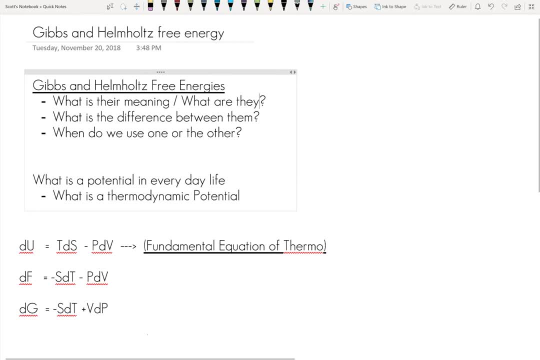 My name is Scott Smith and I'm going to answer a few questions about the Gibbs and Hemholtz free energies. First, what is their meaning and what are they? Second, what is the difference between them? And third, when do we use one or the other To discuss? what are they? we need to talk first. 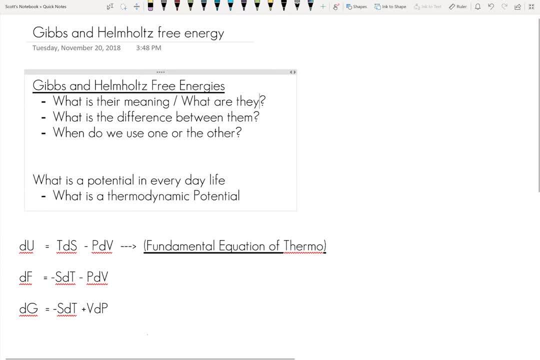 about an everyday potential in real life. So a potential that you might be fairly familiar with- or at least I hope you are- is gravitational potential. So if I raise a box to some height or I change its height, I have given it gravitational potential, energy. Similarly, 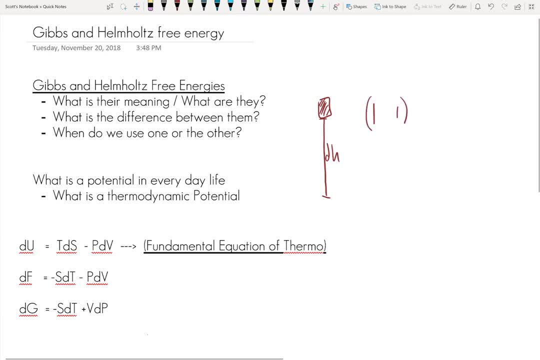 if I have an electron and I have it in a wall socket, one side might be positively charged and the other side might be negatively charged And this electron might have a tendency to migrate to the other side. if I but connect those two sides Similarly, the box would fall if I were. 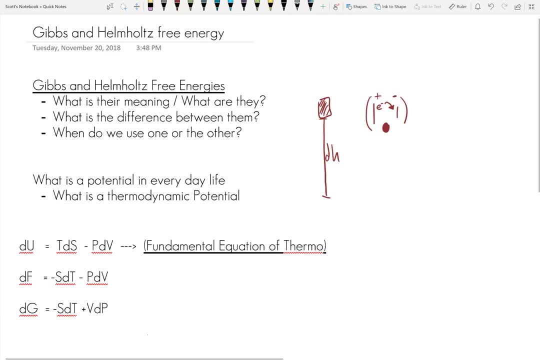 to let go of it, And the energy would then be released, usually in the form of a gravitational potential into heat, but it would also be vibrations and in sounds and other stuff like that. And so these two potentials, gravitational potential and electrical potential, they tell us. 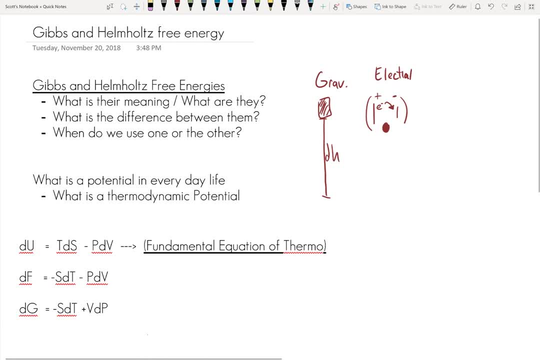 how our system has stored the energy, And we can learn things about how the system will evolve by minimizing these various potentials. Similarly, we have a system that has stored the energy, And we can learn things about how the system will evolve by minimizing these various potentials. Similarly, we have a system that has stored the energy. 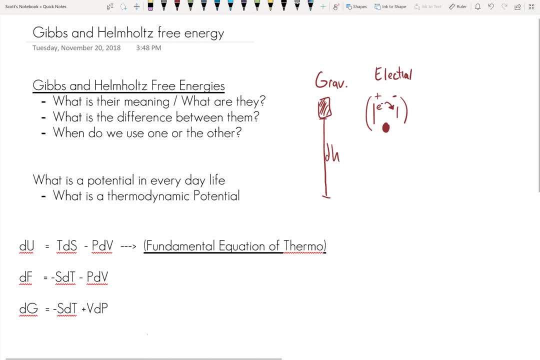 And we can learn things about how the system will evolve by minimizing these various potentials. And we can learn things about how the system will evolve by minimizing these various potentials. And these thermodynamic potentials are useful in a number of different situations, Because we first have looking here at this equation for the change in internal energy from the 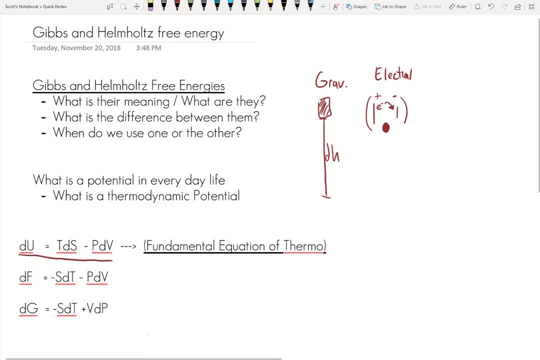 fundamental equation of thermodynamics. we have this heat term, which is both of these terms here, Q, and we have the pressure-volume work term, which is negative pdV. Further I should have written: uh, this other work, or W squiggle. I'm just going to refer to other work as double W squiggle. 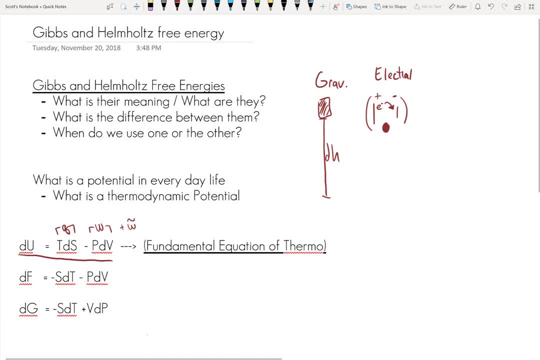 And these other forms of work might include a stress, strain work or, you know, a battery reacting. There's all sorts of different types of work that you can you can talk about And in different situations, when we might have, you know, chemical work from charging a battery. 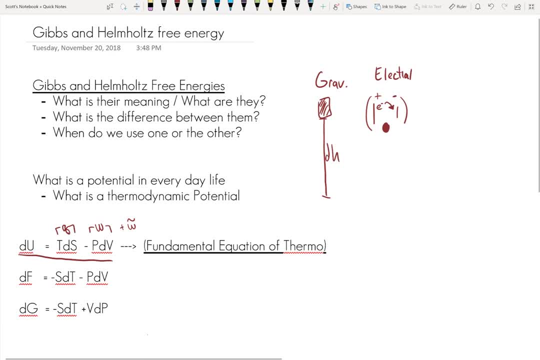 we might be interested in relating that to it's the change in chemical- sorry internal energy. But that brings us to our next question is: when do we use these different potentials? And I should say Helmholtz free energy and Gibbs free energy, just like internal energy, are also thermodynamic. 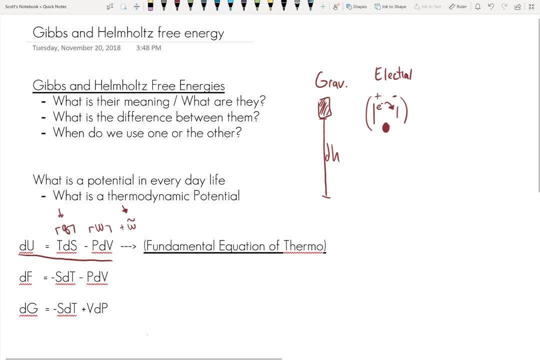 potentials. So when do we use one or the other? and it comes to this idea of natural variables? when I'm talking about a change in gravitational potential, or when I change, rather, when I change the height of an object. I've changed the height of an object. I've changed the height of an object. 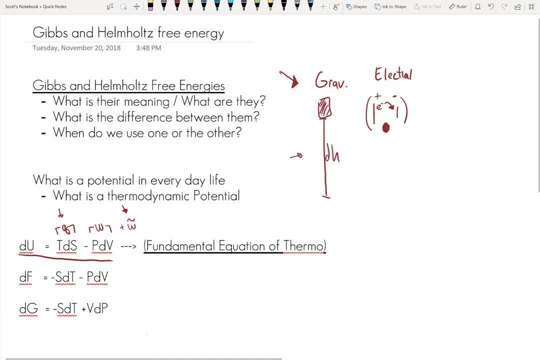 I've changed its gravitational potential And thus the natural variable of the gravitational potential is height. But when it comes to internal energy, if I knew how the entropy changed and the volume changed, then I could relate how the internal energy is changing to those two changes. 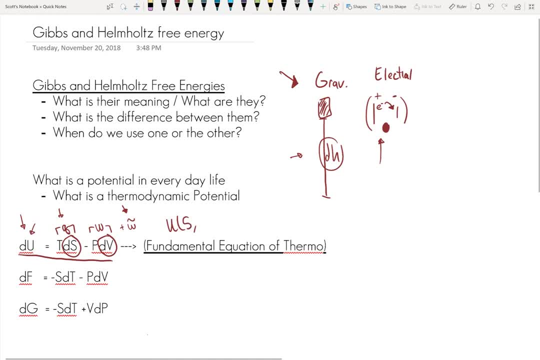 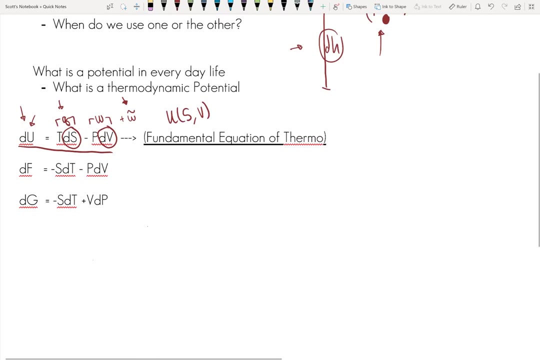 And so we see that internal energy, its natural variables are entropy s and volume v, And so if we knew how a system behaved with entropy and volume, then it would be very easy to track the internal energy. Often, however, it is much more convenient to talk about pressure, volume and 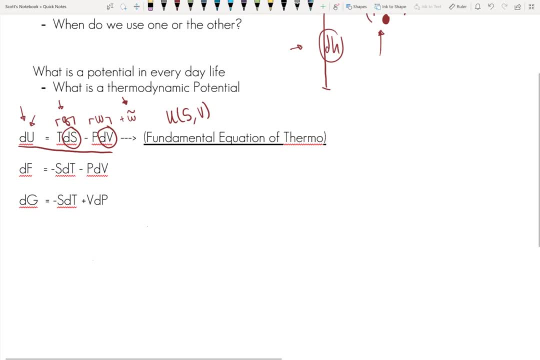 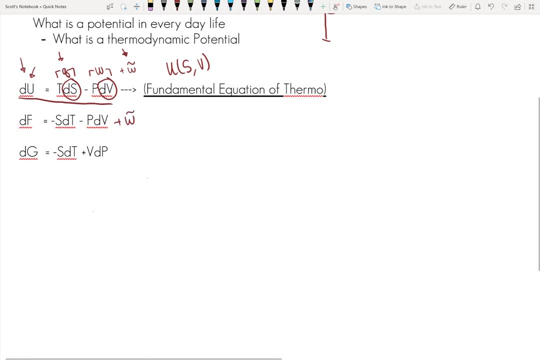 temperature And the two thermodynamic potentials that are most frequently used to talk about pressure volume and temperature relationships, and I should mention these other forms of work often, or pressure volume work, the potentials that are used to relate those things are Helmholtz. 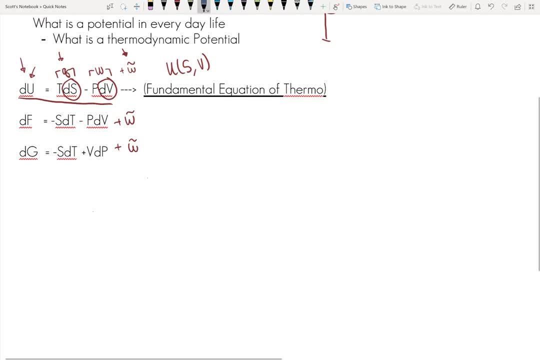 free energy and Gibbs free energy. And, as I'm sure you have already pieced together, the natural variables of the Helmholtz free energy are temperature and volume, And the natural variables of the Gibbs free energy are temperature and pressure. And so in material science we often see, because things are at constant temperature. 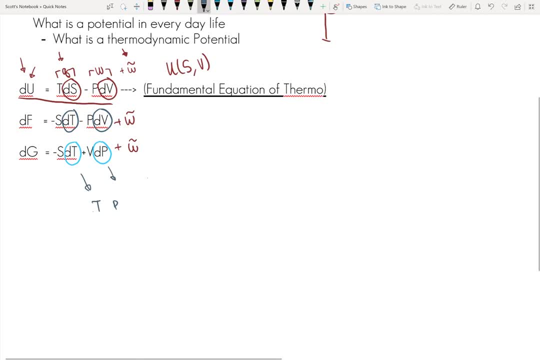 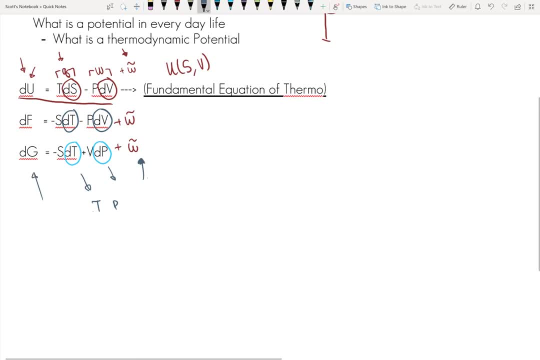